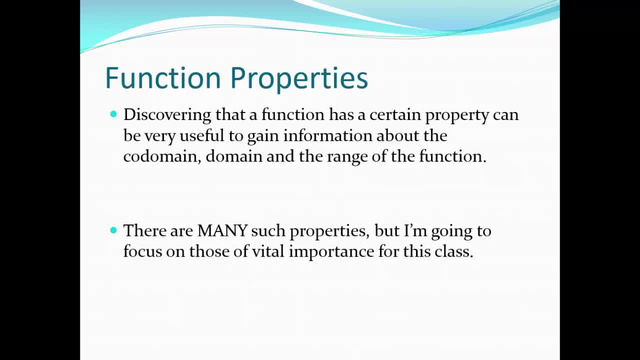 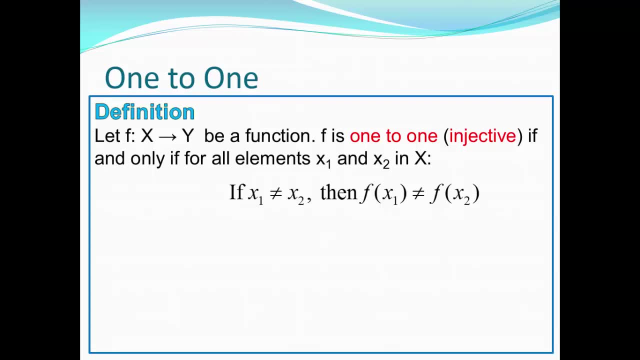 There are many, many, many, many such properties. I'm going to go over a few of them Now. the first one is function. The first one would be one-to-one, So let f be a function going from the set x to the set y. 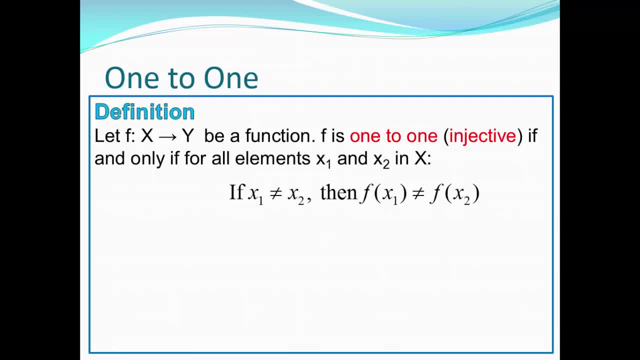 We say that f is one-to-one. Also we say it's injective If and only if for all elements x sub 1 and x sub 2 in the set x, that if the elements x sub 1 and x sub 2 are different, then the outputs f of x sub 1 and f of x sub 2 are also different. 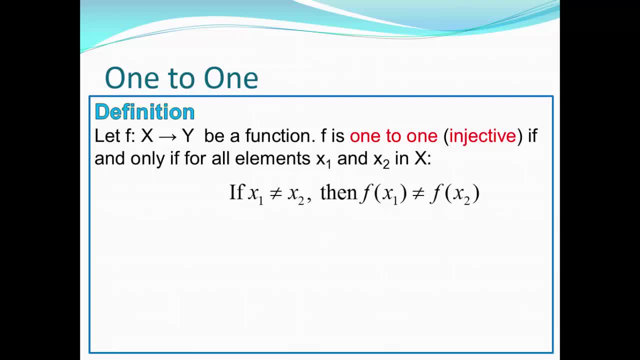 Now, equivalently, if you took the contrapositive, If you took the contrapositive of that statement, it's equivalent to saying that if the outputs are the same, then the inputs are the same. If you want to say in layman's terms that if you give it different inputs, then if the function is one-to-one, you must get different outputs. 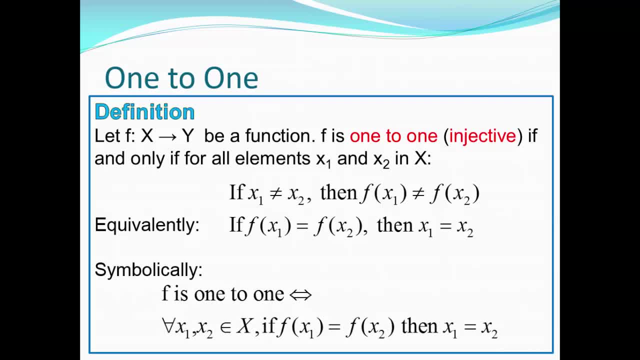 So symbolically we say that f is one-to-one. It's equivalent to saying that for all x sub 1 and x sub 2 in the set x, if f of x sub 1 equals f of x sub 2, then x sub 1 equals x sub 2.. 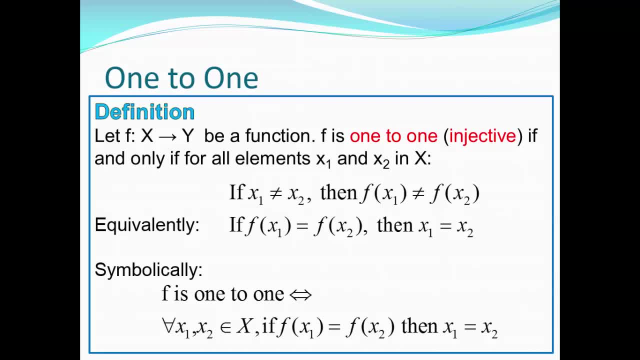 Now the sum Symbolic statement here of one-to-oneness is often the form that we use if we want to show that a function is one-to-one. But in layman's terms we actually use the definition I gave you, that if the inputs are different, then the outputs are different, because it's just easier to say. 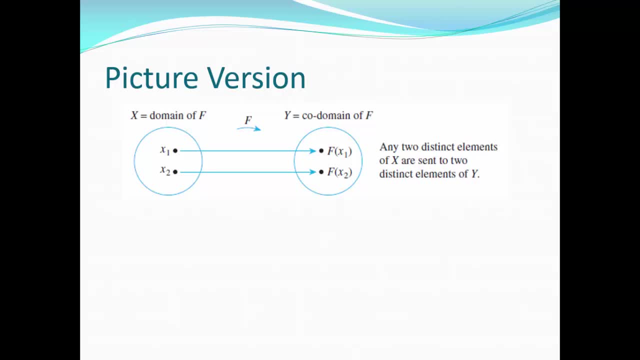 Now here's a picture version of it. This function here is one-to-one. Notice: x sub 1 and x sub 2 are different. So since the function is one-to-one, because I said it is the outputs f of x sub 1 and f of x sub 2.. 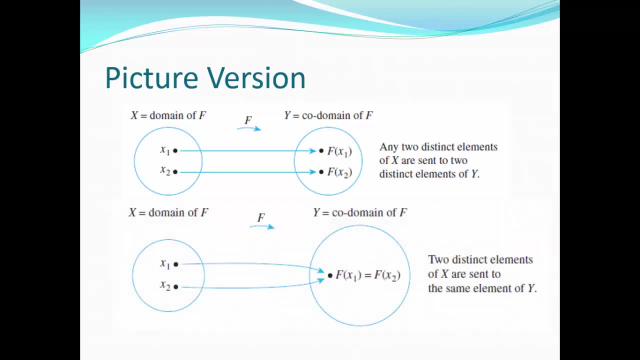 They are different. But if f is not one-to-one, then there are at least two elements. There's at least two distinct elements that their image is the same. That means if f is not one-to-one, it in some way collapses the set x to be something a tiny bit smaller in the set y. 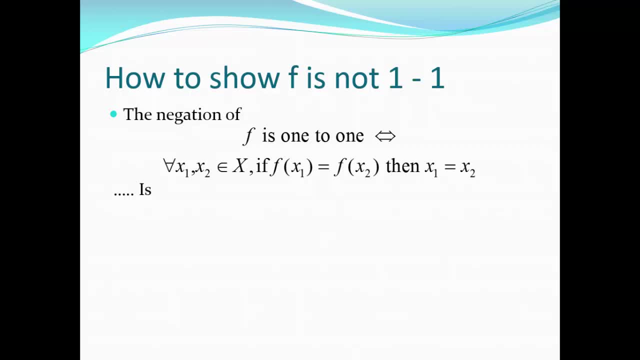 Now, how do you then show that f is not one-to-one. So the negation of f is not one-to-one. So the negation of f is not one-to-one. So the negation of f is not one-to-one. 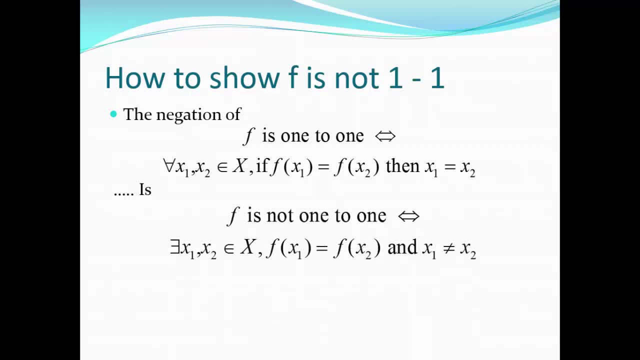 f is one-to-one is Well. if f is not one-to-one, that means there already exist two elements: x sub 1 and x sub 2, so that the function evaluations are the same and yet the inputs are not the same. 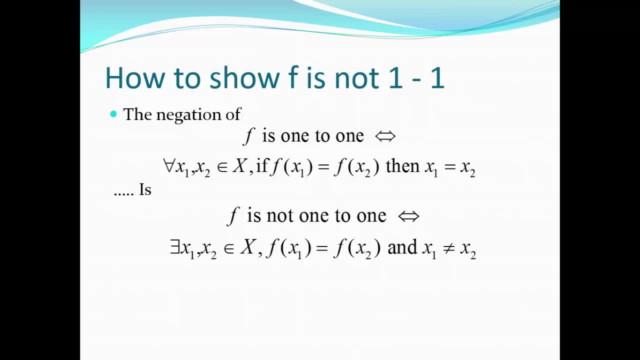 So if you want to show that something is not one-to-one, you have to show an example. You have to give me two elements: x sub 1 and x sub 2, so the function's values are the same for those two inputs. 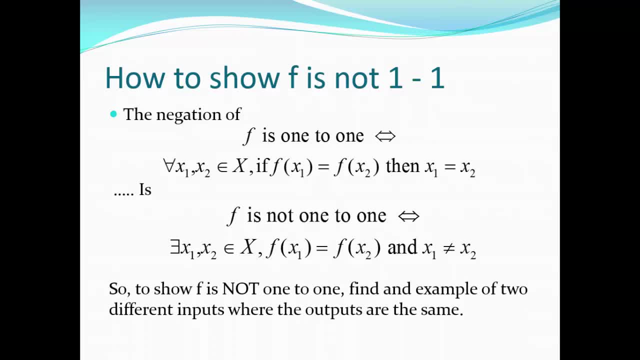 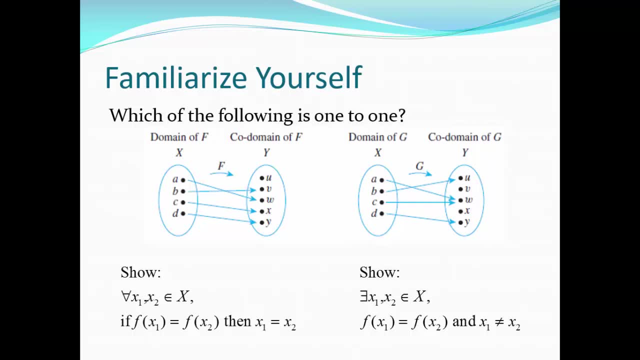 and yet the inputs are different. Now, let's just figure this out, let's just familiarize ourselves. Which of the following two things here is one-to-one? Now, if I want to show something is one-to-one, I have to show that for every x sub 1 and x sub 2. 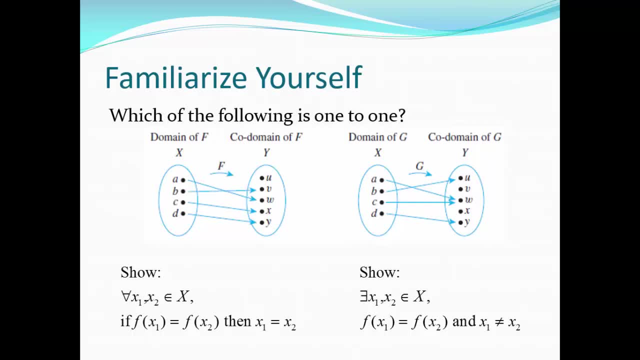 in the set x that if the outputs are the same, then the inputs are the same. If I want to show that a function is not one-to-one, I just show an example, a counter example to the statement that there exists two elements in the domain. 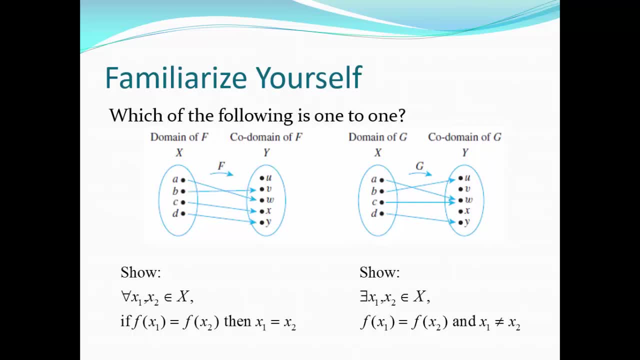 so that their images are the same, and yet the inputs were different. Looking at these two, you can tell that the first one definitely is one-to-one. Notice, one-to-one just does not mean that the range is all of the codemain, because that element u has no image associated with it. 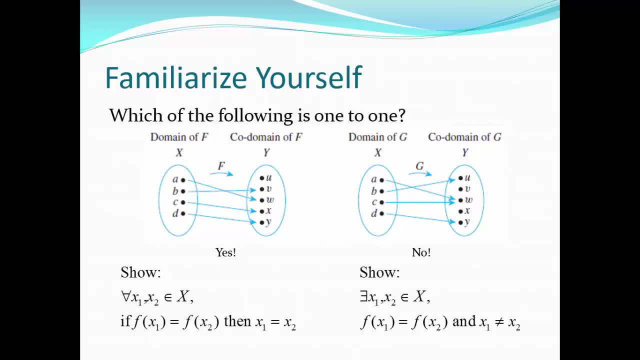 There's no element in x that is mapped to u. But if you look at the second function, g, that function is definitely not one-to-one And the reason is: I can find two different elements in the domain a and c so that their image is the same w. 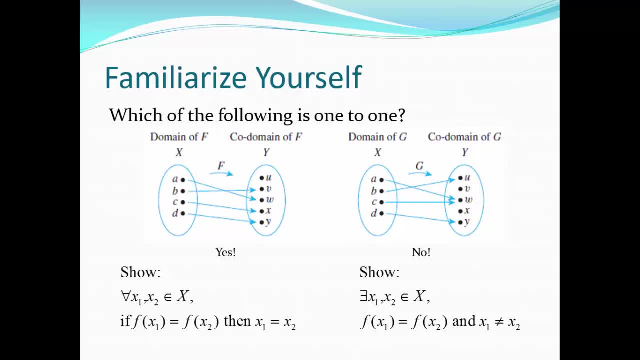 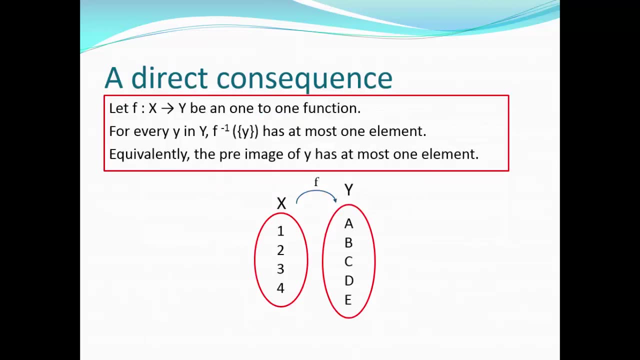 So the images are the same and yet the inputs are different. So that function g is not one-to-one, And I just cited a counter example. Now, as a direct consequence of this thing, if you say f is a function going from x to y, 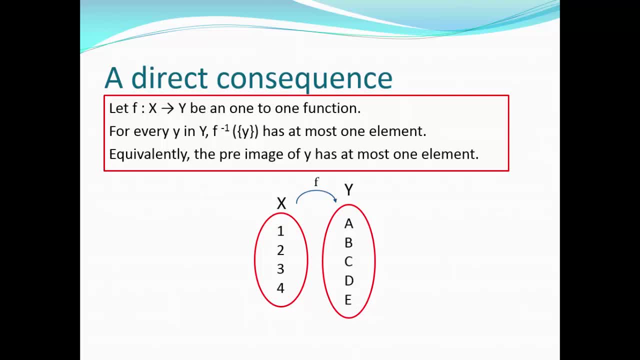 then for every single element in the codemain, the pre-image, the pre-image of that element, has at most one element. It can't have more, Because if it's one-to-one there's at most one thing going to y. So equivalently, the pre-image of y has at most one element. 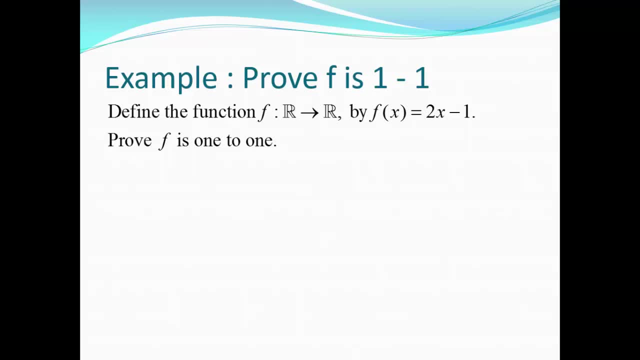 Now let's go ahead and show you how to go improve that a function is one-to-one. I'll just do a really simple example. So define a function. f, going from the real numbers to the real numbers by f of x, equals 2x minus 1.. 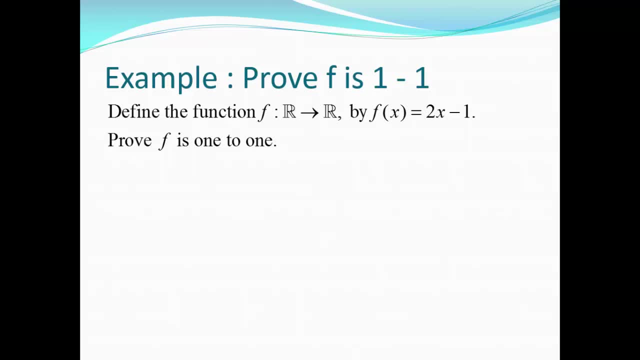 Let's prove that f is one-to-one. Now, to think about that, I have to show then, for any two elements, x sub 1 and x sub 2, in the set x, that f of x sub 1 equals f of x sub 2. 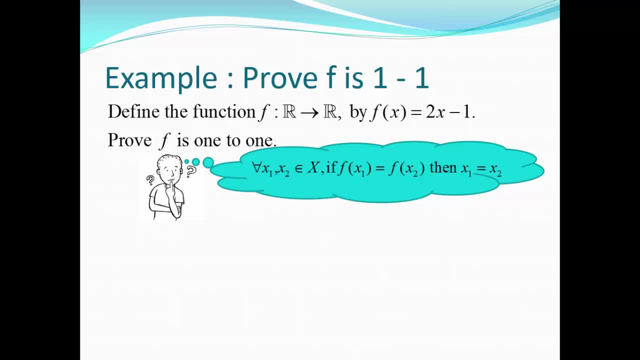 means then that x sub 1 and x sub 2 are the same element. I'm going to do that right now. This is a universal conditional, So with any universal conditional, I start with proof. I then say: let a and b be arbitrary. 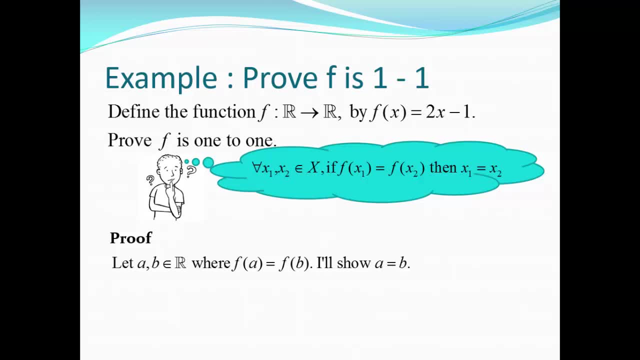 But particular elements of, in this case, the domain in the reals, And I'll also assume that f of a equals f of b. I have to show that a equals b. Now it's just a matter of algebra. So we'll start with. let's assume f of a equals f of b. 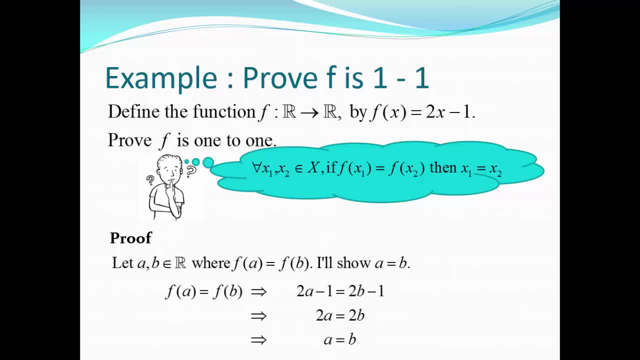 Now that would then imply by the function definition that 2 times a minus 1 has to equal 2 times b minus 1.. But by adding one on both sides that implies 2 times a equals 2 times b. But that would imply, by dividing both sides by 2, that a equals b. 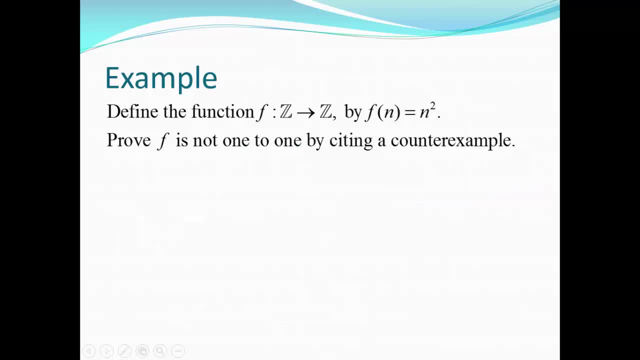 And that's it. That's the proof. Let's define a function, f going from the integers to the integers, by f of n equals n squared. I'll prove then f is not 1 to 1 by just citing a counterexample. So my answer. 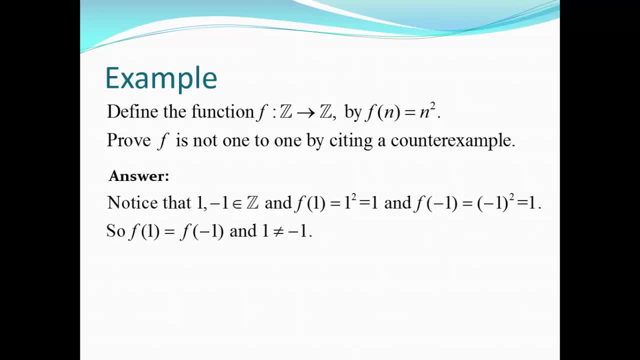 Please notice that 1 and negative 1 are both in the domain of the integers. Also f of 1 is 1 and f of negative 1 is also 1.. So f of 1 equals f of negative 1.. The images are the same. 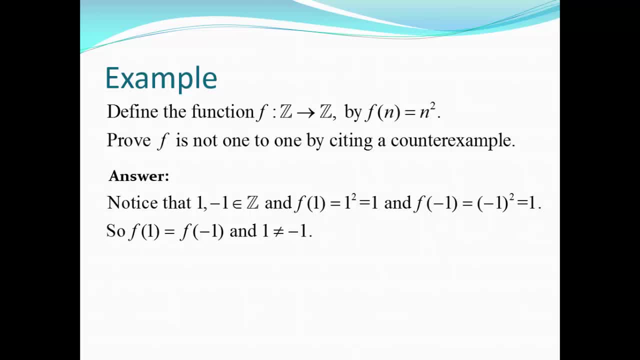 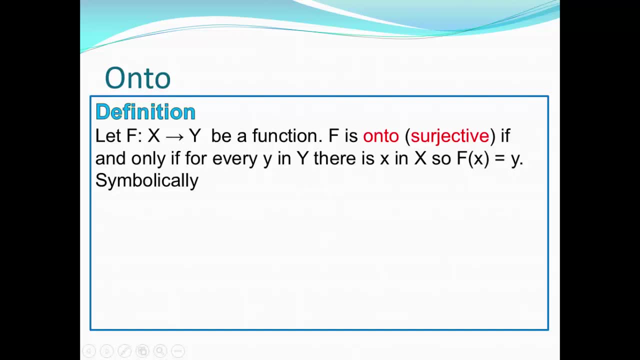 But the input 1 and negative 1 are not the same. This means then f could not possibly be 1 to 1.. Let's look at the second property I'm interested in for functions. It's called onto-ness. Let f be a function from the set x to the set y. 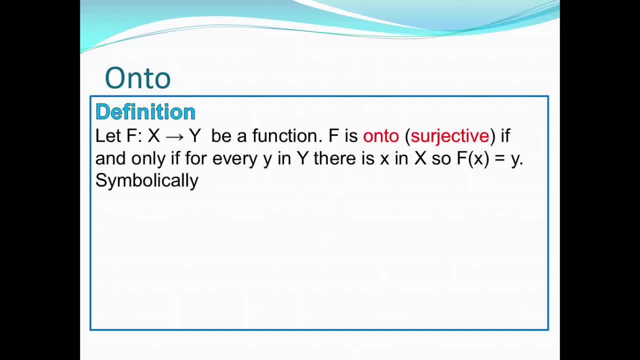 f is called onto or surjective if, and only if, for every y in y there is an x in x, so that f of x is y. Now, symbolically, f is called onto or f is onto y if, and only if, for every y in y there exists an x in x. so f of x equals y. 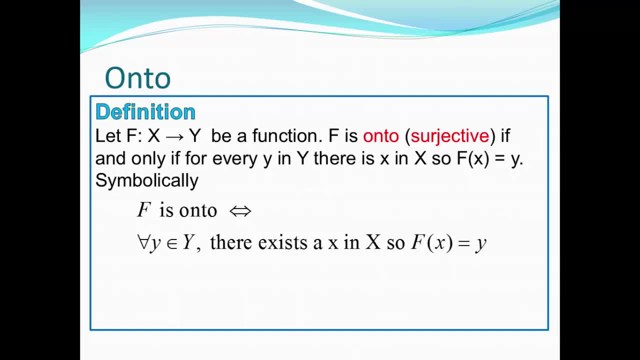 This is a little weird because it has a for every and there exists, So equivalently, this means that f of the set x is y, or the image of the set x is y, or the range of the function is the codomain, or for every single element in the codomain. 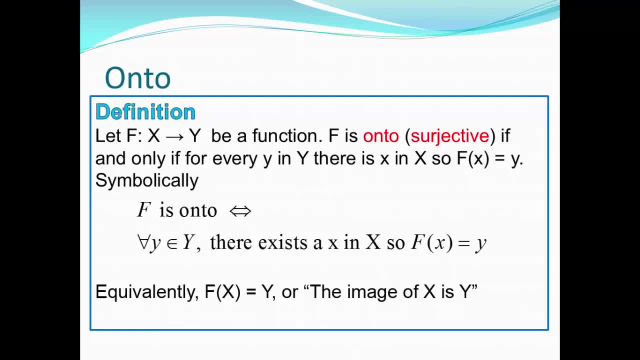 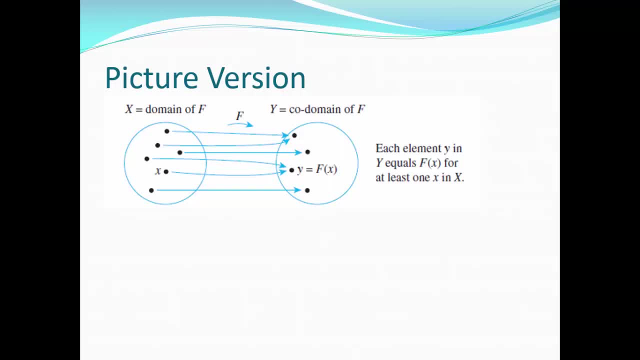 there is an element that maps to it. Lots of different ways to say the same thing. Now here's the picture version. This thing here is onto Notice that every single element in y has an element in x, so that that element x is mapped to that element y. 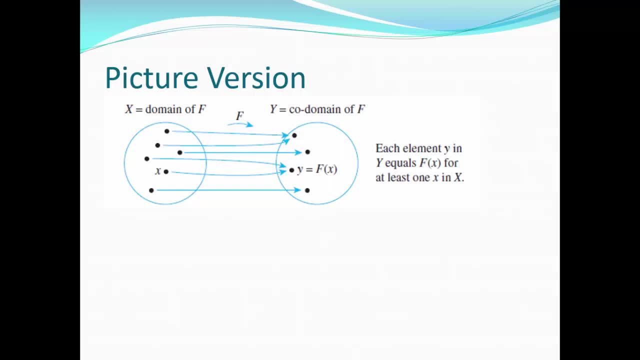 So then every element in y is the image of something in the set x. Now notice, there is at least one element. See that y That's mapped by two things. We don't care, That's okay, It can be mapped by two things. 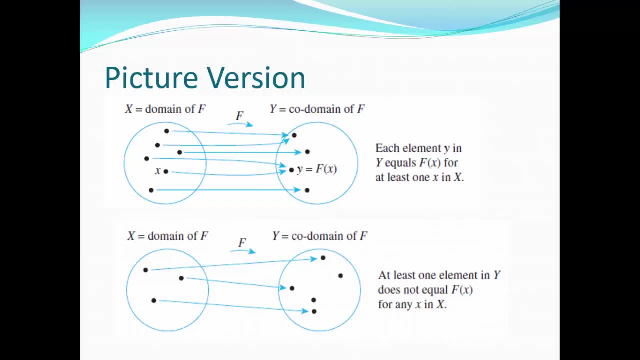 Now here's one that's not onto. There is at least one element. You can probably see it sitting all by itself there on the right. There is one element in y that has no element in x, So the image of that x is that y. 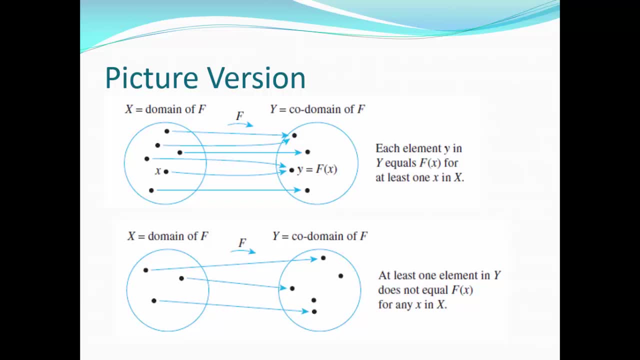 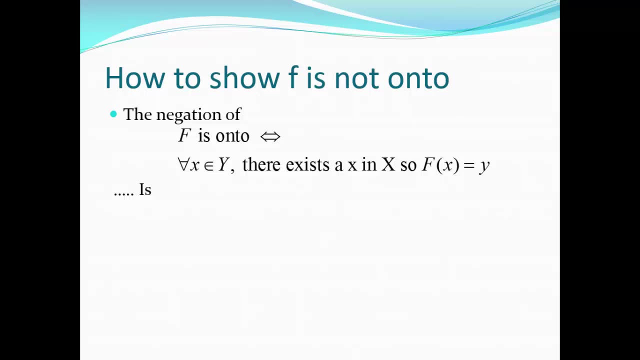 There is an element in the y that has no print image. So now, how can you show then a certain function is not onto, You just have to do the negation. So if f is onto, if you want to take the negation of that, 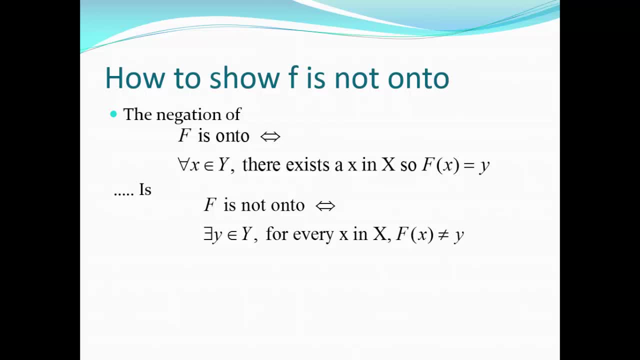 then f is not onto implies that there exists a y, so that for every x in x, that f of x is not y. Now, that's not onto. Now, that's just a symbolic negation. I'll translate it for you, Though. so if you want to show that f is not onto, 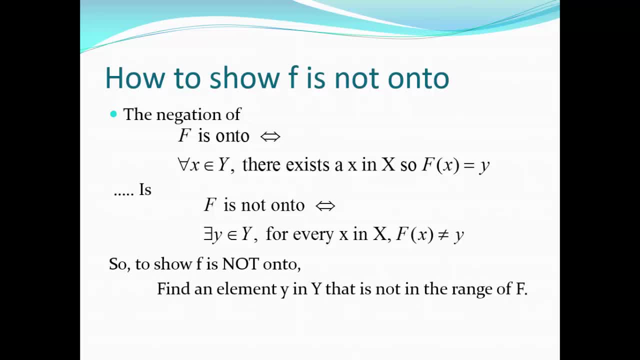 you have to find some element in y so that it is not in the range of f. You can also say there is not an x, whose image is that y? Or you can say that the preimage of y is empty. These all say the same thing. 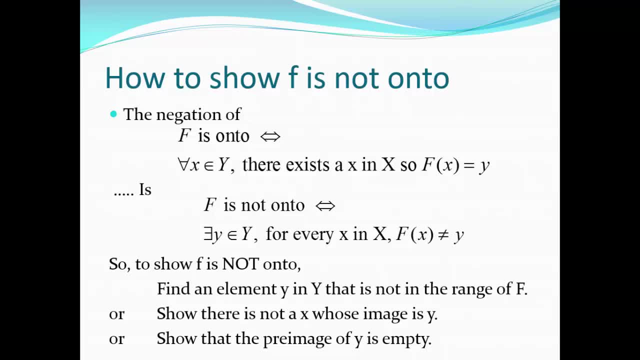 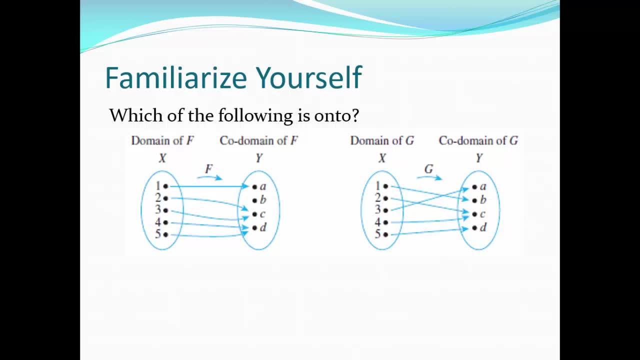 That would mean? then, if any of these are true, it's equivalent to saying that f is not onto. So let's just familiarize ourselves. So here's two functions: f and g. One is onto, one is not. By looking at the two, you can probably tell that the one the right, g. 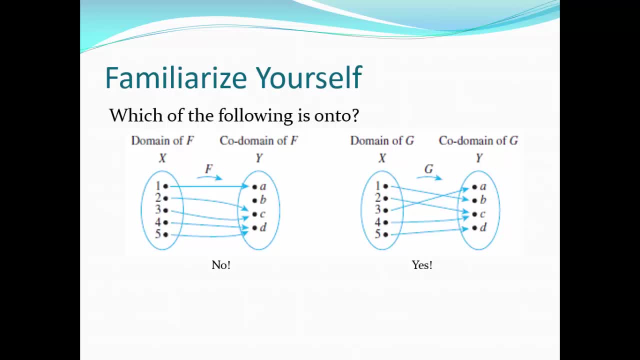 is definitely onto, while f, though, is not. Now, it's not hard to tell, It's not hard to show. If you want to show that something is not onto, I have to show there exists a, y. in this case it's b. 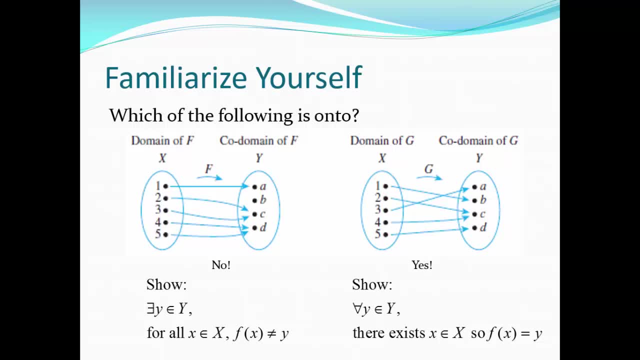 so that for all elements in x, f of x is not y. So if you take the image of 1,, 2,, 3,, 4, or 5, none of those would be b when you look at the image under f. 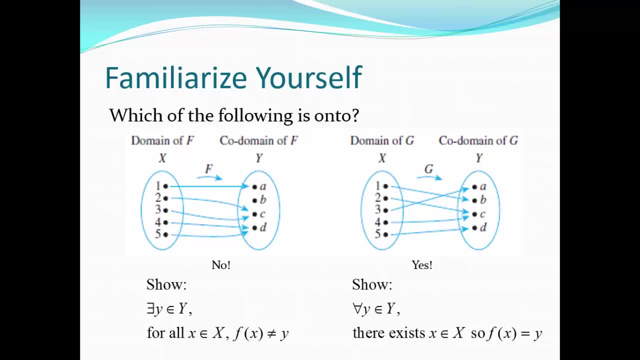 Compare that to the function g. If you take any element in y, there's at least one element in its preimage. That means for every element there's at least one element in x that's mapped to that element in y. So, for example, if I were to pick b in y, 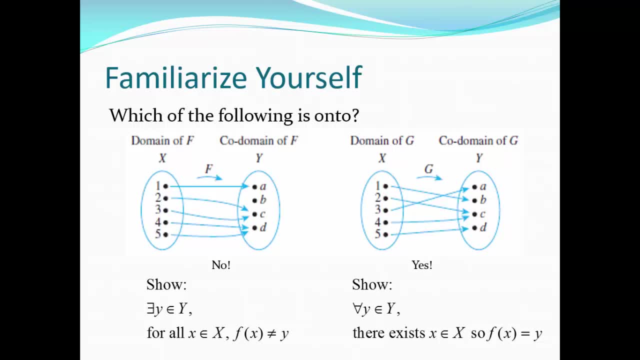 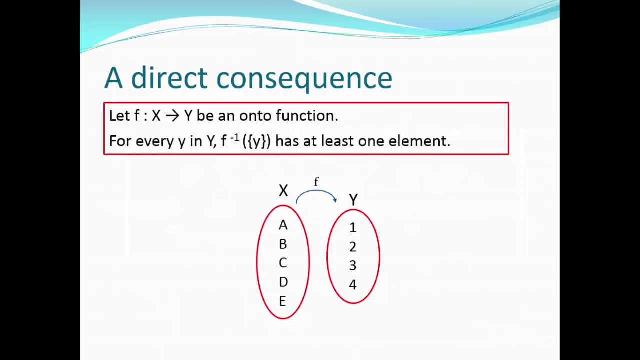 there's an element 1 in x, so that g maps 1 to b. Now, as a direct consequence of this, it's literally just reading right from the definition pretty much If you say f is a function going from x to y. 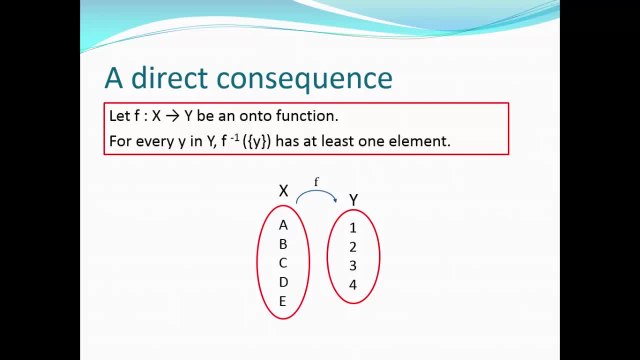 and it's an onto function, then for every y in y the preimage function of the set y has at least one element, Because if it's onto, then for every element in y there's at least something in its preimage. 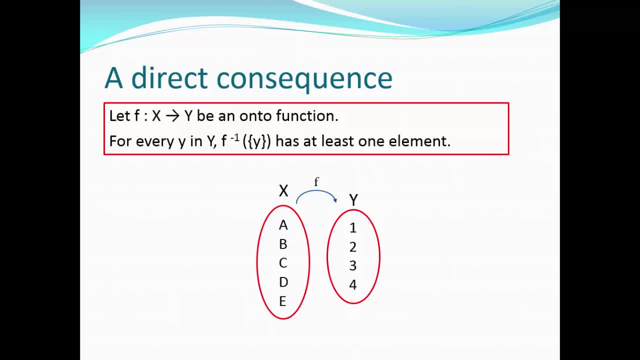 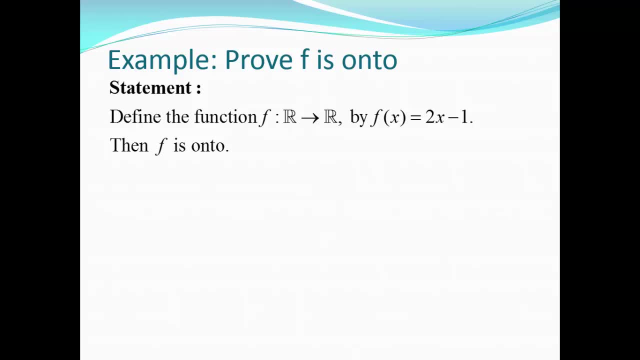 And that's exactly what that says. Okay, Now I'll show you how to prove that a certain function is onto. Let's define a function going from the reals to the reals, so that f of x equals 2x minus 1.. 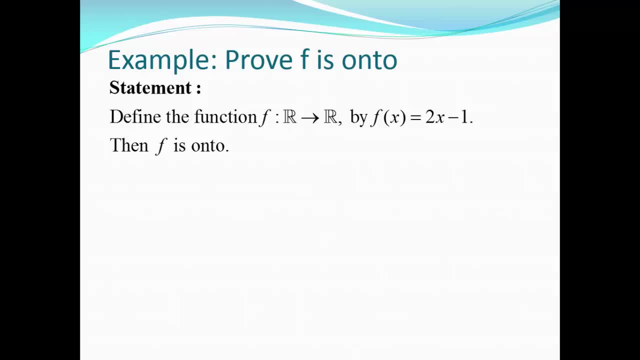 I think you remember I showed this one before Then. f is onto. Now to prove something is onto is typically more difficult than proving something is 1 to 1.. The reason is it's partly an existence statement. In this case you have to prove that for every y in the reals. 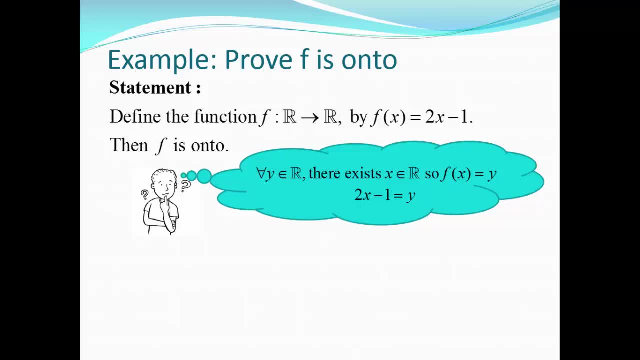 that's every y in the codomain. there exists an x in the domain, so that f of x is y. To translate that: if you give me any y, I have to find you an x, so that 2x minus 1 is y. 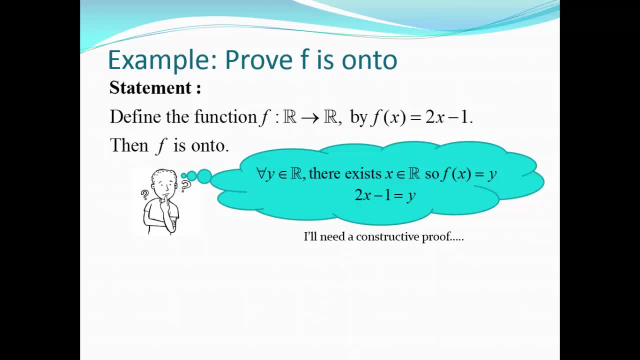 This isn't a constructive proof. I have to show you this element in the domain Which I'll call x, so that f of x is that y. Now, a common way to do this is to sort of start with what we want and work backwards. 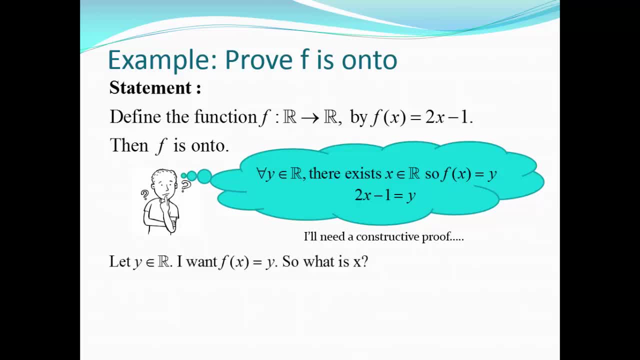 So I have something in the codomain, I'll call it y. I want to find an x, so that f of x is y. So I'll just write down: f of x equals y. But if f of x equals y, I know what f of x equals. 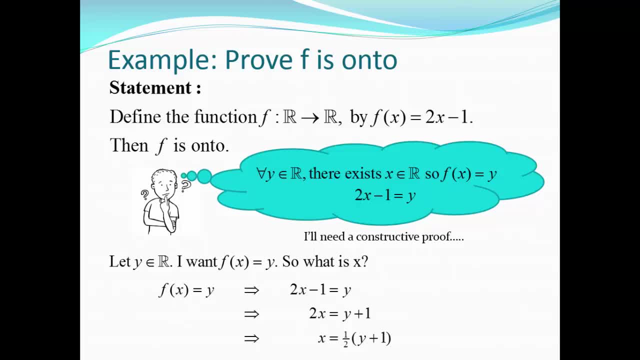 It's 2x minus 1.. That means 2x minus 1 is y. I'll just find all the x's, I'll just solve for it, if it's possible, And here, because this is all algebra, I just add 1 to both sides. 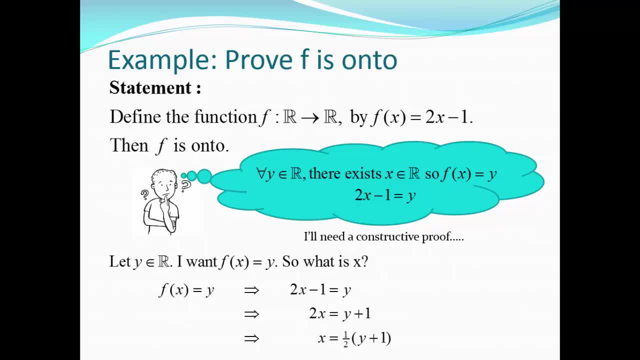 and then I divide by 2 to get whatever this element is. It must be 1 half y plus 1.. I'm now ready to do my proof. I'm just going to take the scratch work I just showed you and actually write down the argument. 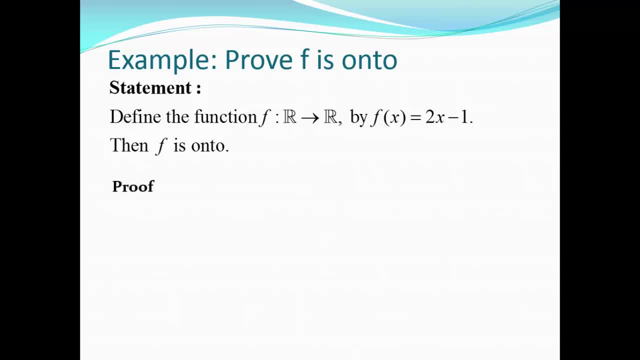 Now. so the actual form of proof, this time Proof. Let y be something in the codomain. Define x to be 1, half y plus 1.. Please notice that, since y is a real number, when I add 1 to it and then divide by 2,. 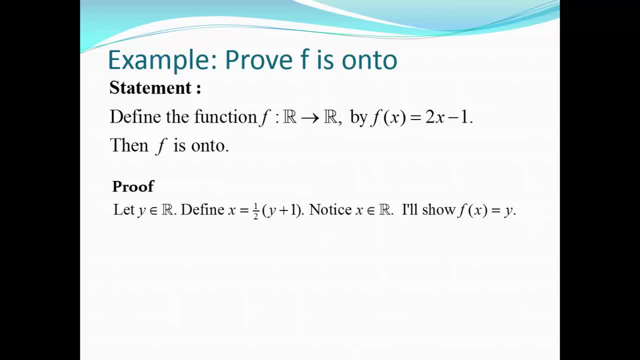 it's also a real number. So then this thing I just defined happened to be something in the domain. I'll now show that f of that element, x, is y. Alright, so then just cranking up the definition: f of x is f of. 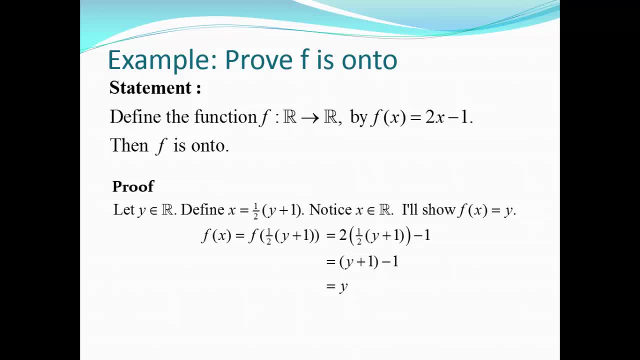 1 half x plus 1.. But f takes anything, doubles it and subtracts 1.. So then f of that expression should be 2 times the expression 1 half y plus 1 minus 1.. Now just doing the algebra then. 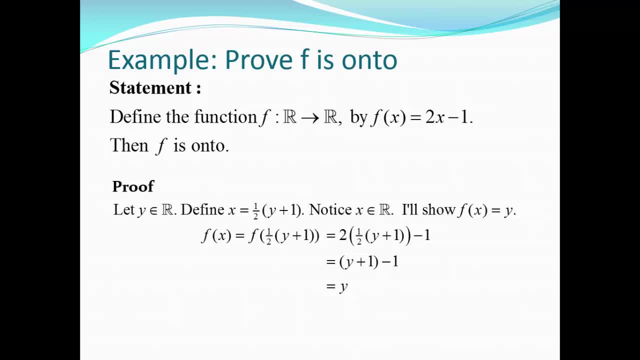 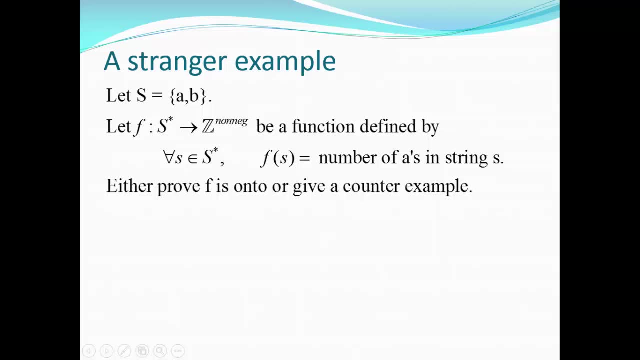 the 2 and the half cancel. I would then have y plus 1 minus 1.. That's y. So f of x indeed is y, f is onto. Alright, here's a stranger expression, For example, looking at a function defined on a set of strings. 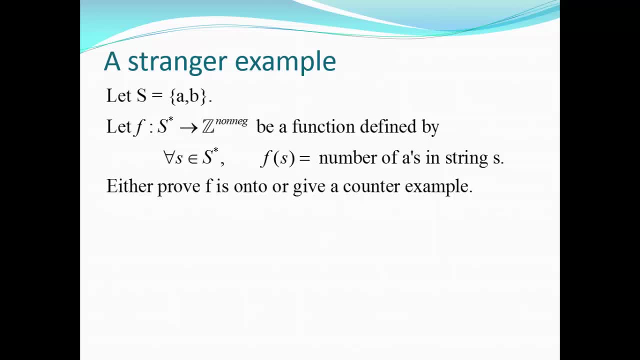 So let s be the set. Let f be a function going from the set of all finite strings- Remember that's the s star and s is called the alphabet. Going to the non-negative integers be a function defined by: for every string of a's and b's. 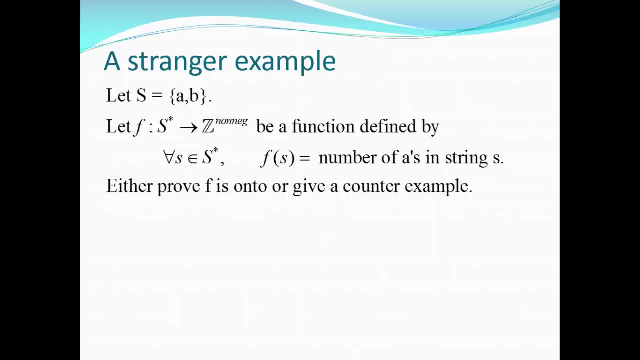 That's finite, f of s will equal the number of a's in the string s. Now you remember me defining this one before. I'm either going to prove that it's onto or I'm going to give you a counter example. Now, this problem is more challenging than the other ones. 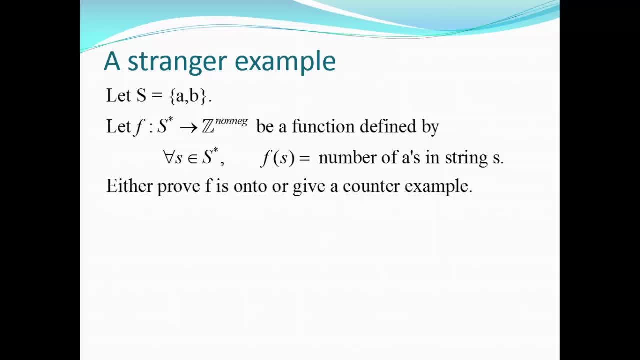 because I didn't tell you what to do. You have to figure it out yourself. A good way to attack these problems is to be positive about things. Assume it is and try to figure out what the proof would look like If at some point you stumble. 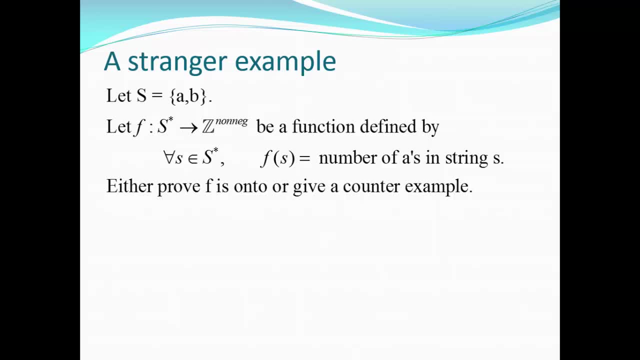 well then, maybe that means it's not true, and you try coming up with a counter example. So I'm going to try to be positive about things. So I have to show, then, that for every n, which is a non-negative integer, there exists a string. 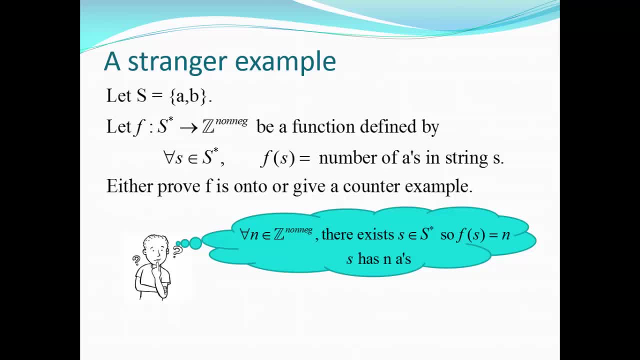 so that f of s is n. Now translating, f of s is n. f of s is the number of a's in the string. So that means s the string of a's and b's will have n a's. So can I show you. 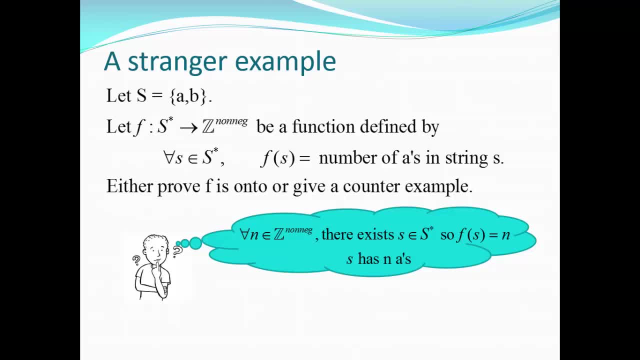 that if you give me any integer I can find a string of a's and b's so that, f when I map that string to the set of non-negative integers, that that string will have n a's. Well, yeah, easy, That wouldn't be hard to do. 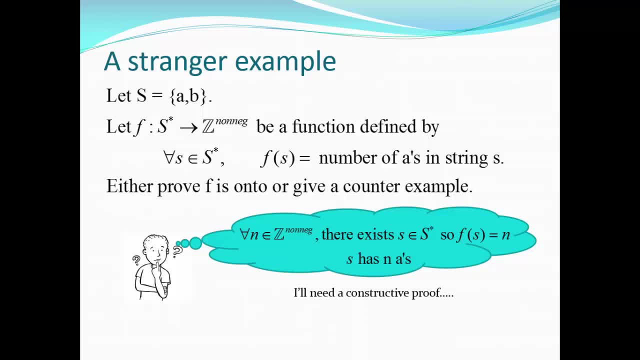 It's just a proof by construction. I'll just make that string for you. So here's the proof Proof. Let n be any non-negative integer, So it could be 0 and so on. Define s as the string of n? a's. 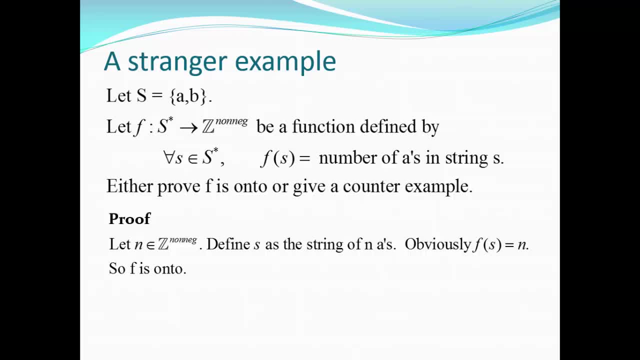 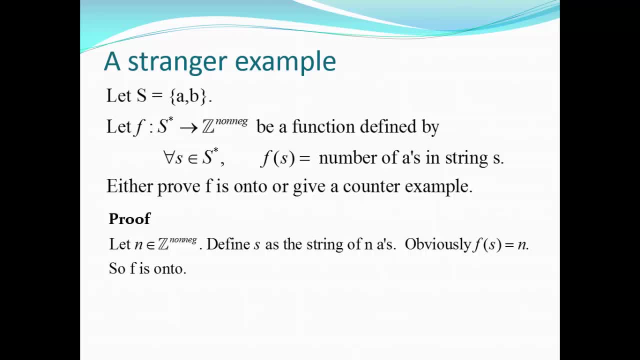 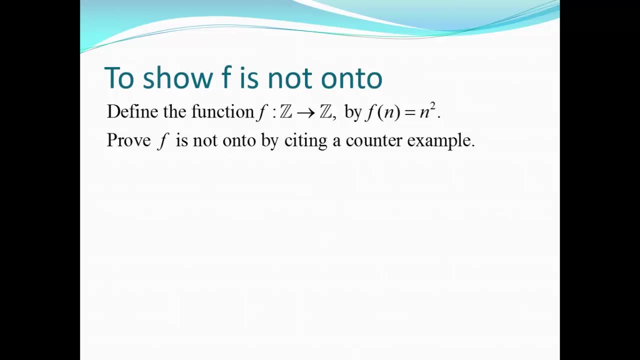 the number of a's in s? Well, but s has n a's, So yeah, f of s is n. There's nothing to do. That function definitely is onto Now, how to show something is not onto Well. once again, I'll. 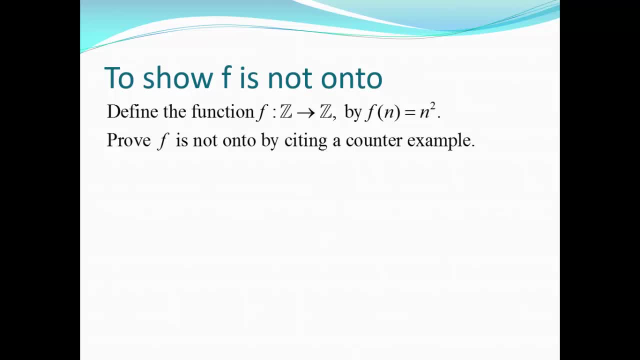 show that it's either onto or I'll set a counterexample Here. I'll show you a counterexample. I have to show you that there's something in the code domain, so there's no element in the domain, so its image is the element I started with. 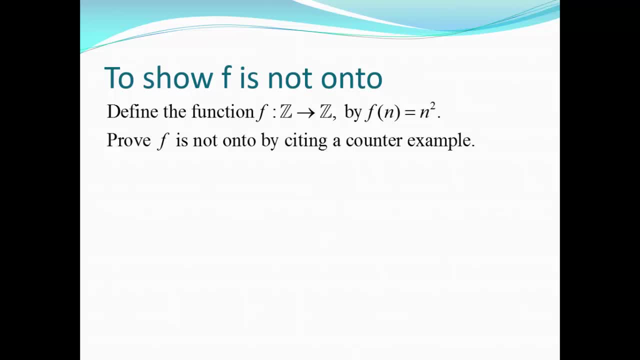 So is there an element in the code domain whose preimage is empty? So, as a counterexample, I need something that when I square it, that it's an integer, But when I come back that it's not an integer. So let's see. 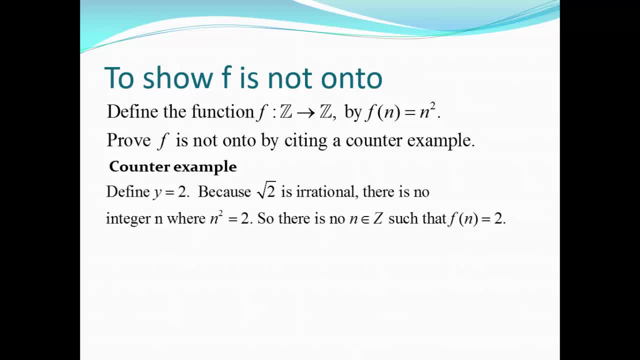 Look at 2.. 2 is an integer, but notice, though, the square root of 2 is irrational. That means that, since that's not irrational, the square root of 2 is not an integer, because integers are irrationals. Therefore, there is no integer. 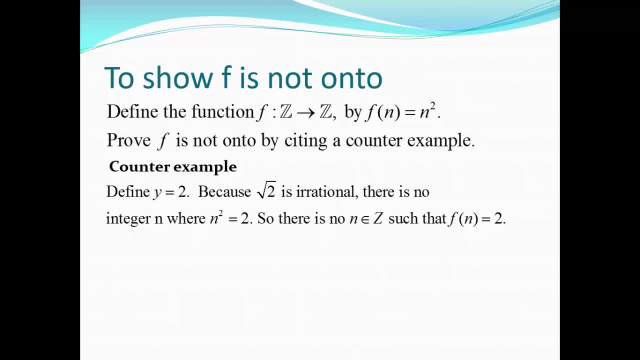 so that n squared is 2.. That means then there's no integer in the domain, so that f of n being n squared is 2.. That's it. This function is definitely not onto. It is not onto the set of all integers. 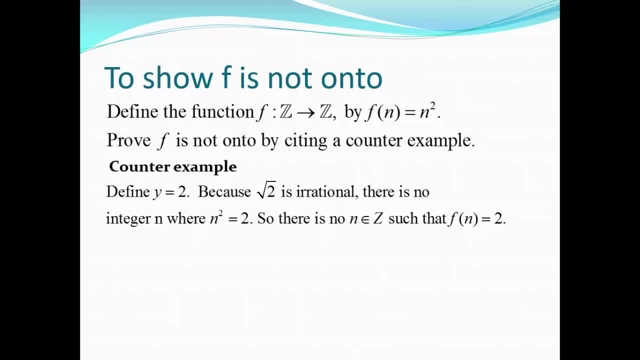 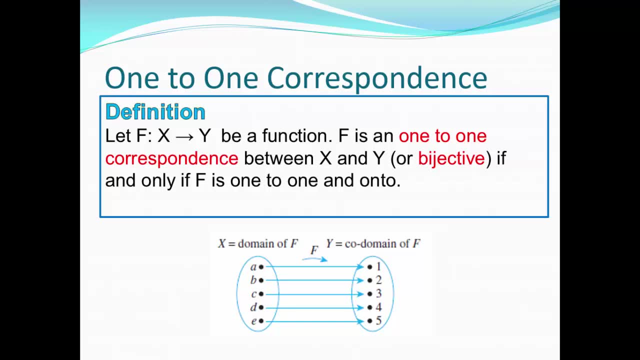 There are things that are integers, that are not squares of integers. So now, if we get lucky, our function will be 1 to 1 and it will be onto That's given a special name. So let f be a function going from the set x to the set y. 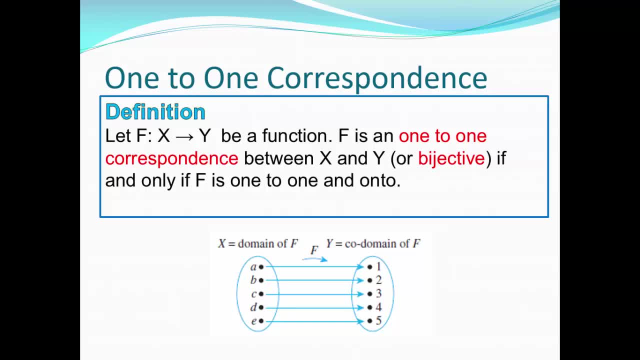 If f is a 1 to 1 correspondence between x and y, or it's called bijective. if, and only if, f is 1 to 1 and it's onto So notice, then if I want to show that f is a bijection or it's a, 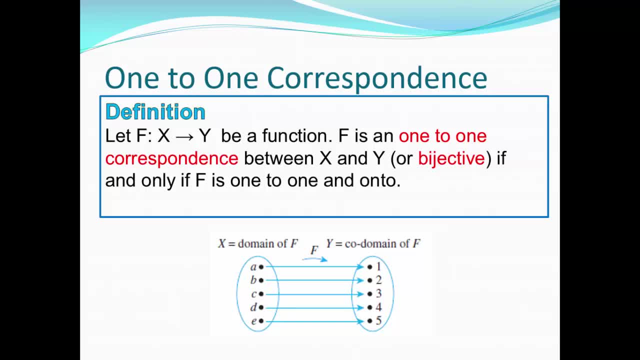 1 to 1 correspondence. I have to show it's onto and I have to show it's 1 to 1.. So there's actually two little proofs I have to do. Here is a function going from two different sets. where that function is. 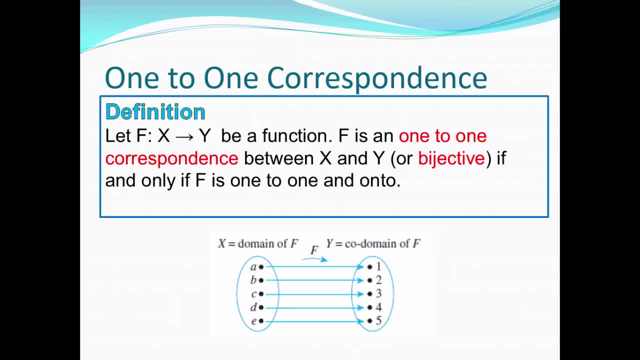 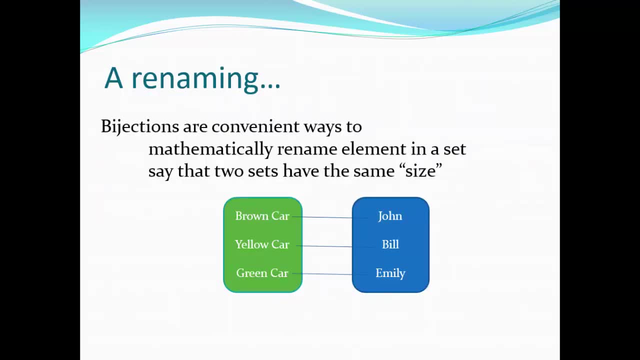 a 1 to 1 correspondence. Now you need to have an idea of what kind of 1 to 1 correspondence does. So the easiest way to view a 1 to 1 correspondence is: it's a way to rename elements. All it does is it takes. 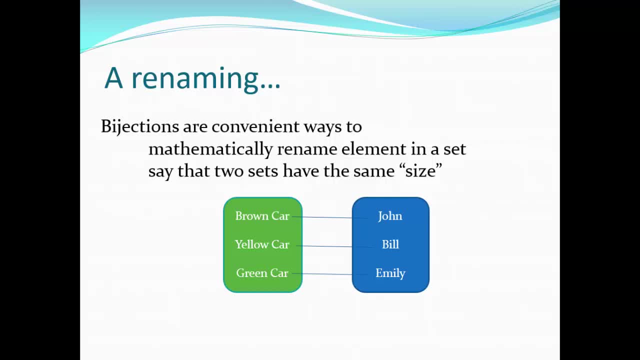 every element in the first set and it gives a name to it. It assigns a new name to it from the second step. So the brown car could be called John, the yellow car could have been called Bill and the green car could have been called Emily. 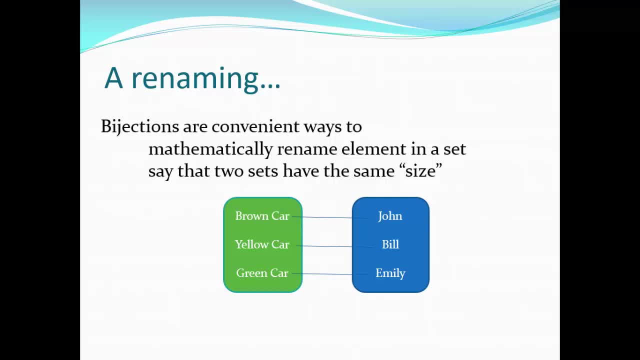 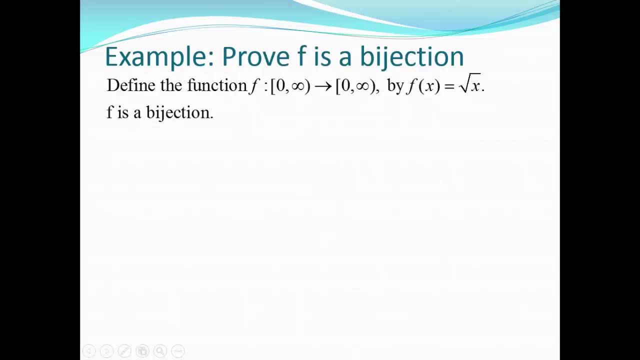 So if I ever said, hey, I want to take John out for a ride, everybody knows that means I'm driving the brown car. I'll show you how to prove that a certain function is a bijection. So let's define a function. f, going from the non-negative reals to the 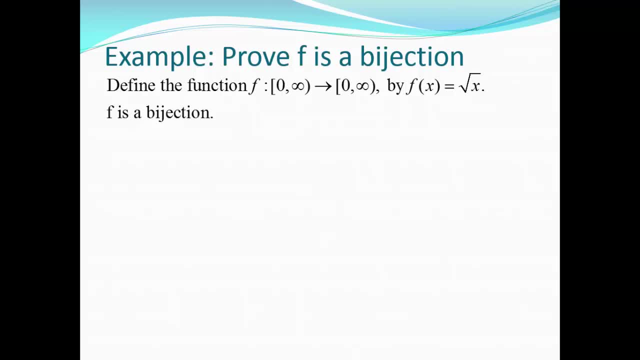 non-negative reals by f of x equals the square root of x. f is therefore a bijection. You can also say that f is a 1 to 1 correspondence between these two sets. To prove that, I have to then show you that f is 1 to 1 and it's. 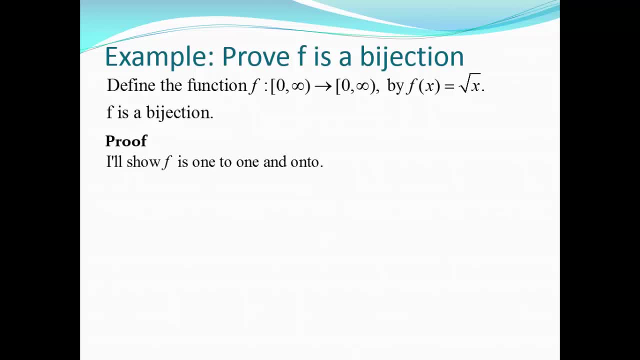 onto. So there's two small proofs in here. I have to show that f is 1 to 1 and I have to show that f is onto. I'll do the onto-ness first. So let's take something in the codomain, I'll call it y. 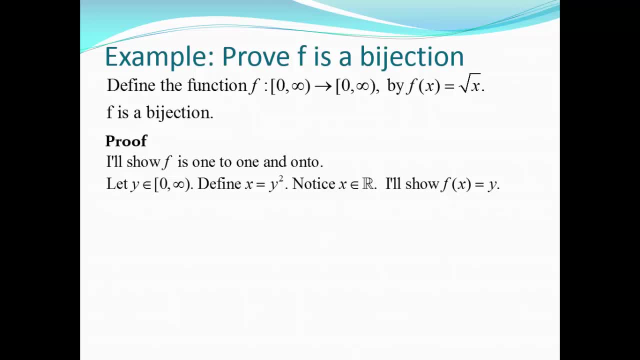 So y, then, is a non-negative real. I'll then define, because I have to show there exists something. I'll define something in the domain. So let's define x to be y squared Now, since y is a real number, when you square that real number, 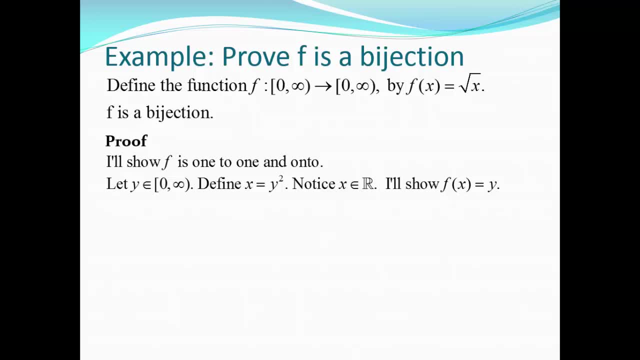 it's also a real number. so x is a real number. So x is in fact something in the domain. I'll now show you that f of x equals y In this case. this is just a matter of banging up the definitions, banging out all the algebra. 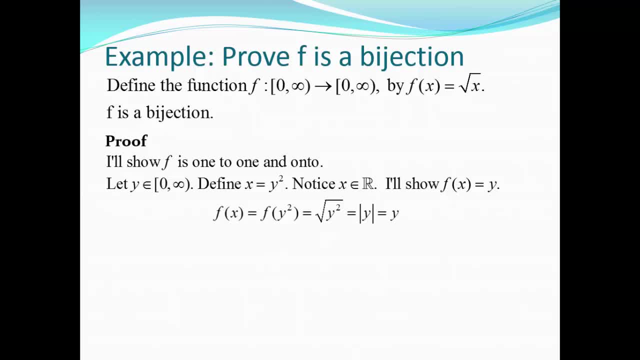 So let's see f of x. that equals f of y squared. But that would then equal, by the definition of f, the square root of y squared. But if you remember you may not, the square root of y squared is actually not y, It's the absolute value. 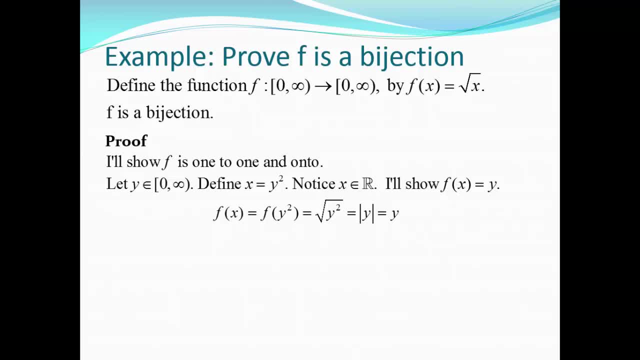 of y, But y was a non- negative real. So then the absolute value of that non-negative real is that non-negative real. So the absolute value of y in this case is just y. That shows that f is onto, because f of x is y. 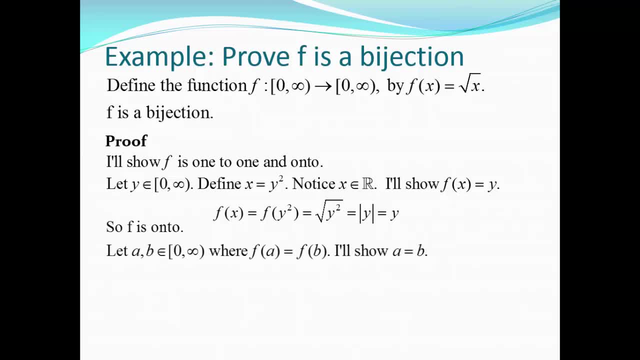 Now I'll do one-to-oneness. So let's say we have two elements in the domain. I'll call them a and b, Because I don't like calling them x sub 1 and x sub 2.. I'll call them a and b. 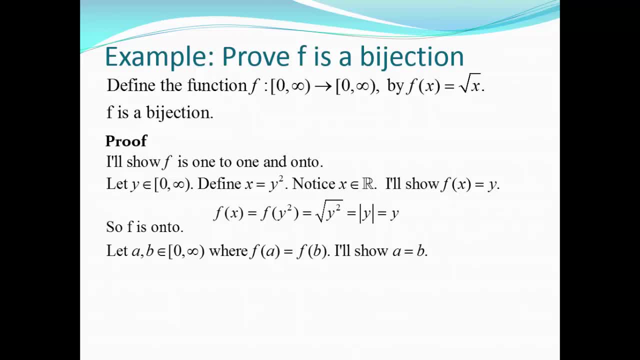 And I'll assume f of a equals f of b. I'll prove to you then: a equals b. So it's just a matter of algebra. Let's start with: f of a equals f of b. By the definition, that would then mean the square root of a equals. 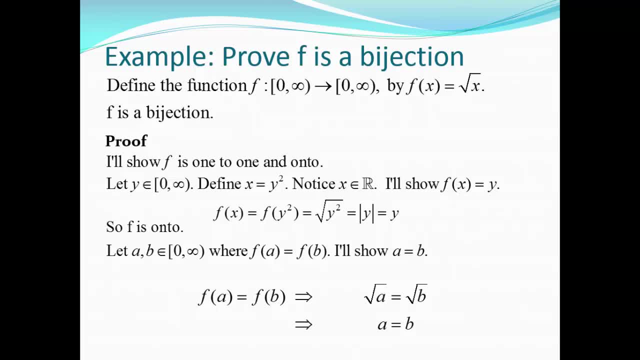 the square root of b By squaring both sides. that means a equals b. That shows that f is one-to-one. So f is indeed one-to-one and onto That means f is a bijection. That's the proof, Pretty straightforward. 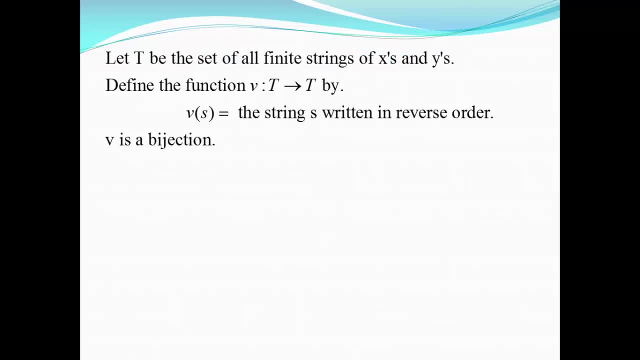 Let's try it again with a more difficult example. Let's try it again with a more difficult example, This time: no algebra, Let t be the set of all finite strings of x's and y's. Now, if I wanted to, I could have said: 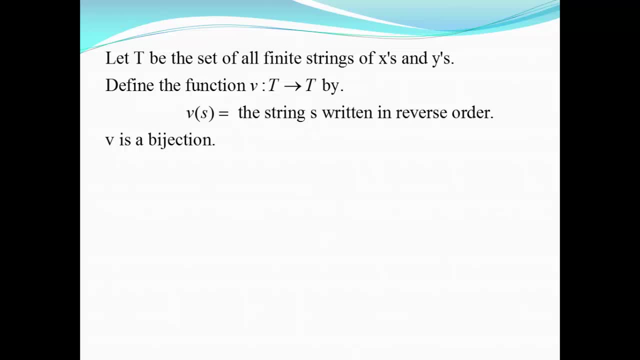 let s be the set x and y, Then t would be the set s star, Because s star is the set of all finite strings of x's and y's. But I won't do that, So then let's define the function v going from this set of finite strings. 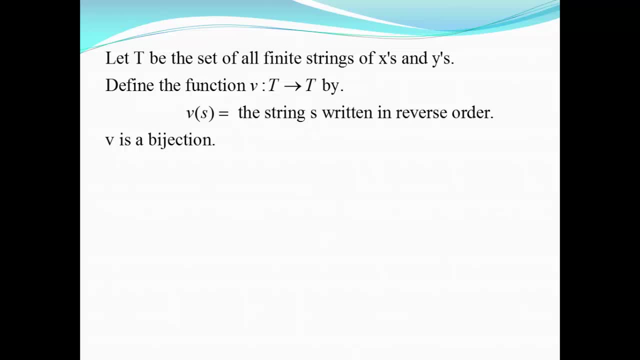 of x's and y's back into the same set. The function will take any string of x's and y's that's finite and will take that string and write it in reverse order. It just reverses it. I claim that v is a bijection. 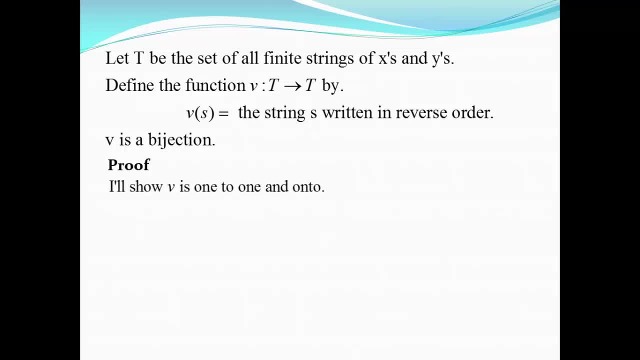 To prove that I have to prove two things. I have to show it's one-to-one and onto. I will take care of the onto-ness first, because that's usually the harder one. So let's take any element in the code domain. 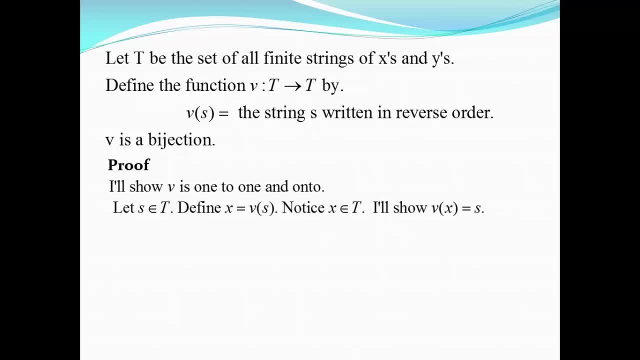 So that's some string that's finite and has only x's and y's. Let's define another string which is found by taking my set s, my string s, and reversing it. So x will be the reversal of the string s. Well, since 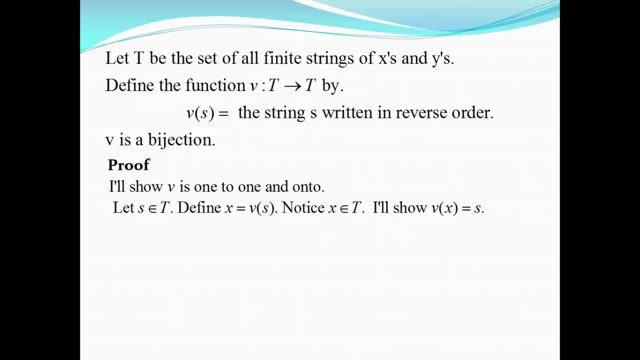 the string s is just a bunch of x's and y's. when you reverse it, it's still a bunch of x's and y's. So then this string is in the set t. So now I'll show them that the function mapped to this string 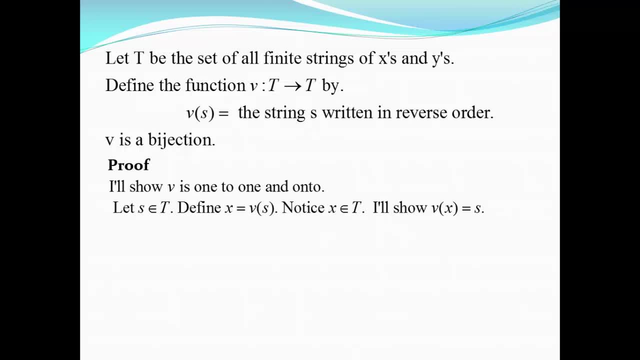 will then give me the original string s. It's just a matter of bouncing through the words. So v of x would be v of v of s, But v of v of s. each time you do a v, you do. reversal of the string. 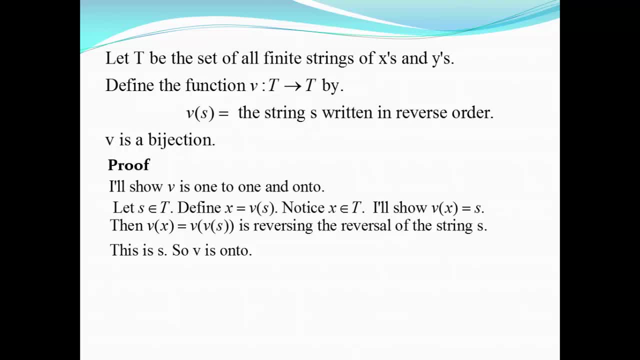 So this is reversing of the reversal of the string s. Well, when you do that, you get the string s back again. So of course, v of x is s, So v is onto. That's it Now. I'll do one to oneness. 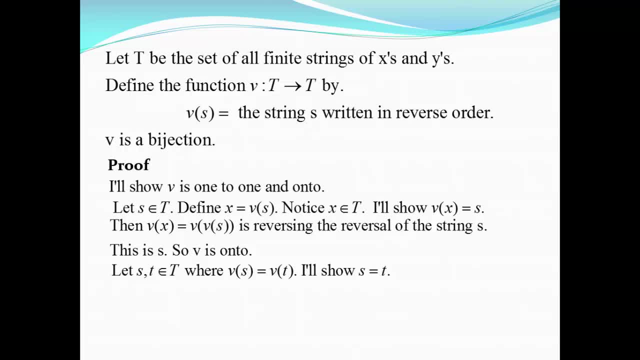 So let s and t be two strings in the set of all finite strings of x's and y's. Let's assume then v of s is v of t. I'll show the two strings: s and t are equal. Well, but if v of s equals v of t, 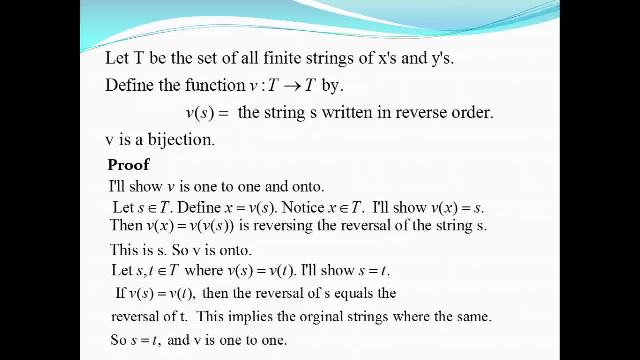 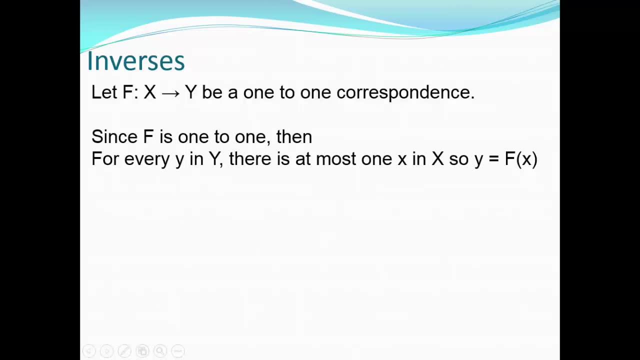 that means the reversal of s equals the reversal of t. Of course that implies then that the original strings are the same. So that means then s and t have to be the same string. That means v is one to one. Alright, let's suppose then you have f. 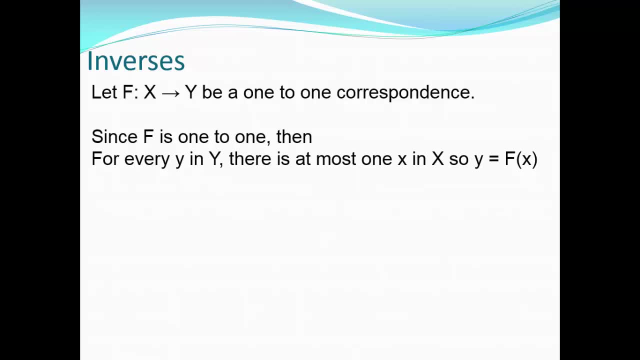 It just happens to be a function from the set x to the set y And it's a one to one correspondence. But that means then f is one to one. So because of that, for every element y in y there is at most one element x in x. 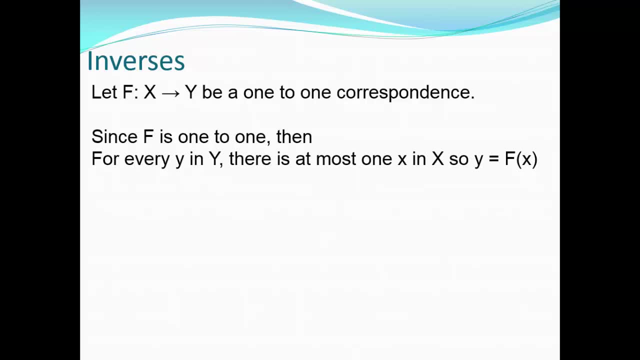 so it's related in some way. But at the same time, since f is onto, then for every y in y there is at least one x in x, So that x and y are related in some way. This is the definition of a function. 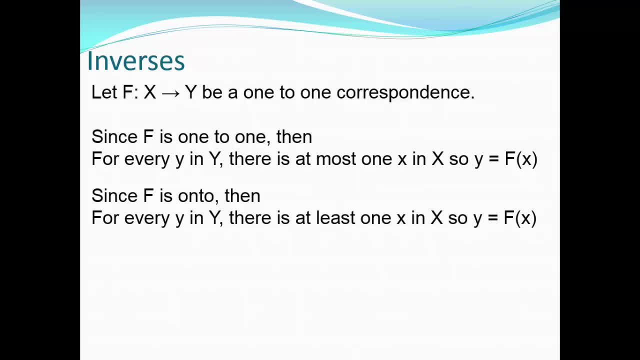 The definition of a function is: for every element in one set you get one and only one element in the other. So then, if f is a correspondence, one to one, correspondence between x and y, there must be for every y a unique element, x in x. That's a function. 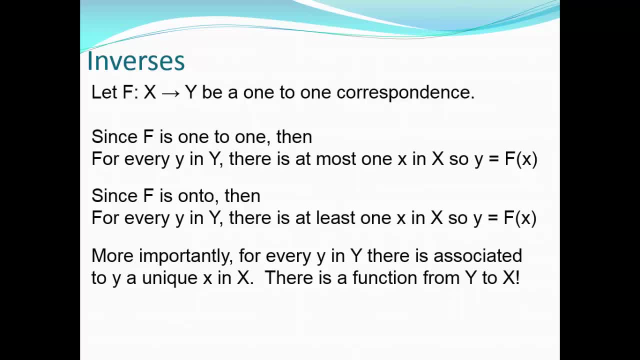 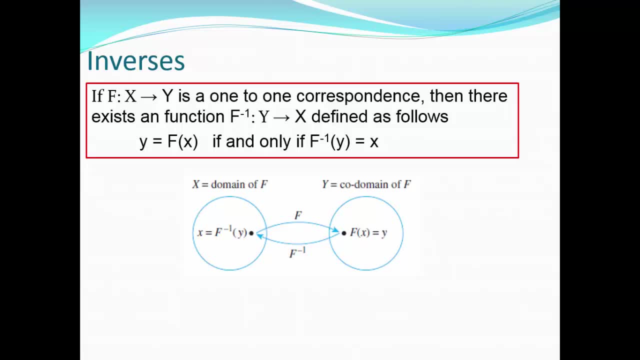 but going from y back to x. That leads us to the definition of inverses. If f, being a function from x to y is a one to one correspondence, then there exists a function f inverse- going from y back to x, defined as follows: y equals f of x. 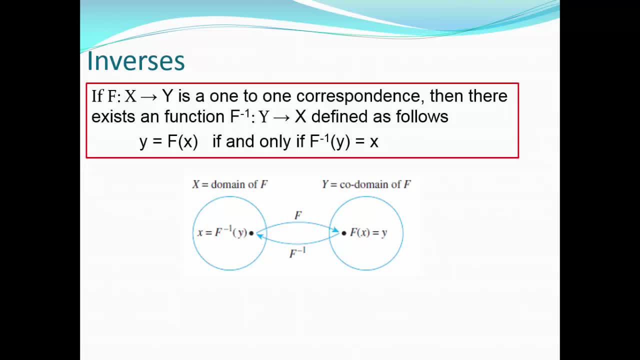 if, and only if, f inverse of y is x. Please notice that by the diagram if you have an element x in the set x, then f maps that to y, but f inverse maps that y back to x. They sort of undo each other. That means 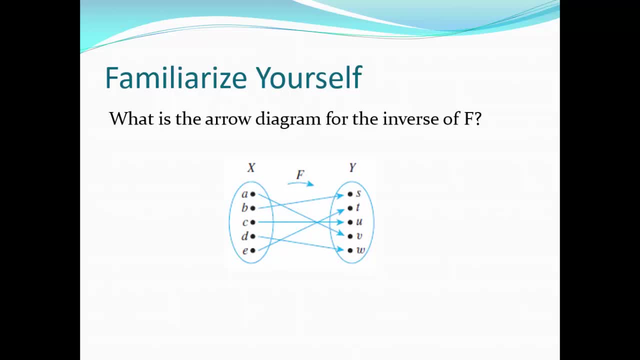 that if you want to. if I told you a function is a one to one correspondence between sets, as this one here is. this function f is a one to one correspondence between the set x and the set y. if I gave you an arrow diagram for that function, it would be. 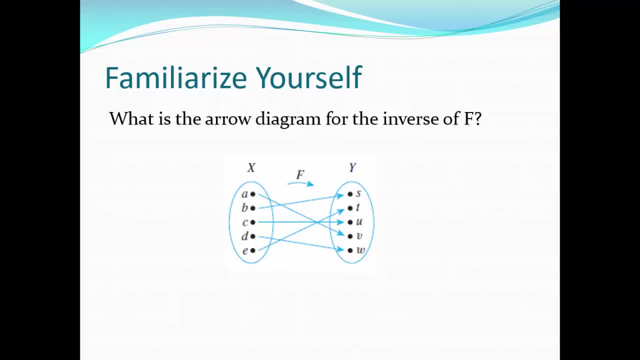 really easy to find the inverse function. All you have to do is just reverse the arrows. So if a goes to v by f, then f inverse maps v to a. It's just the arrow goes backwards. Now that makes it really easy to find inverse functions. 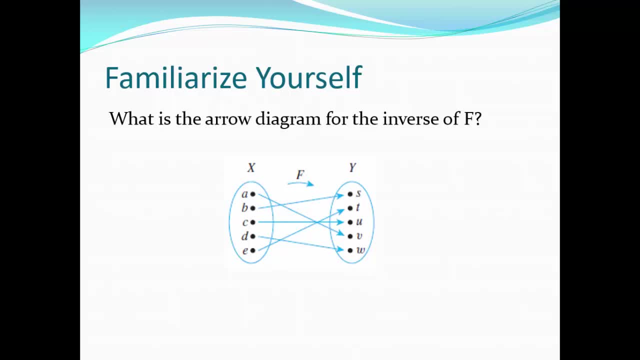 between two finite sets. It's really more challenging, a lot more challenging, if you have a function, a one to one correspondence between two infinite sets. So let's look at an example. I want to define the function going from the reals to the reals. 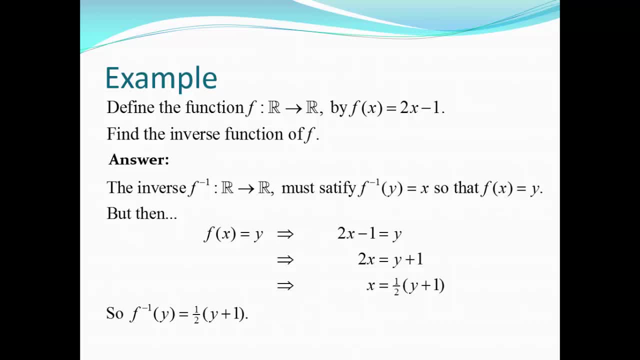 by the function f of x equals 2x minus 1.. Now, in this presentation, I have already shown you that this function is one to one and it's onto, So this function definitely is a bijection. It is a one to one correspondence. 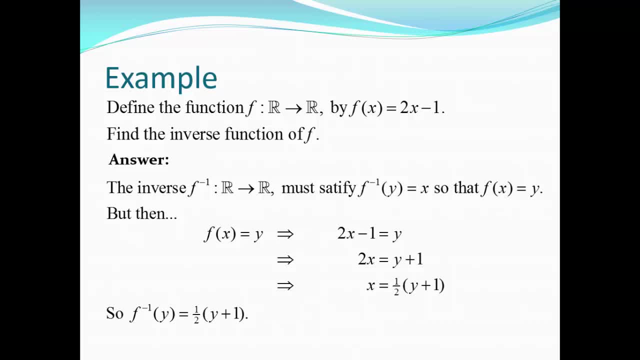 between the reals and the reals, So it has an inverse function. I just want to know what it is. Well, the inverse function is a function, so it has a domain and a codomain. It just so happens, though, that the domain and 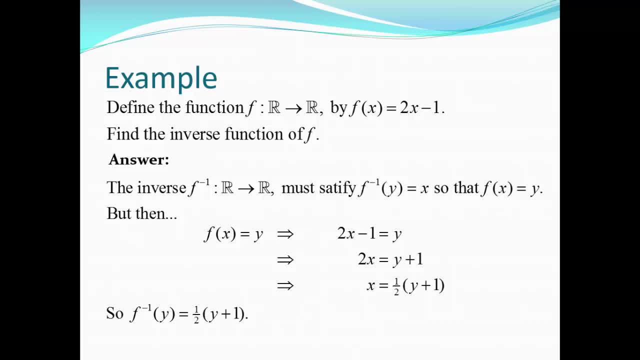 codomain of the inverse are the codomain and the domain of the function. They just reverse. In this case they just happen to be the same sets. So I now know that f inverse must go from the reals back to the reals and it has to satisfy by definition. 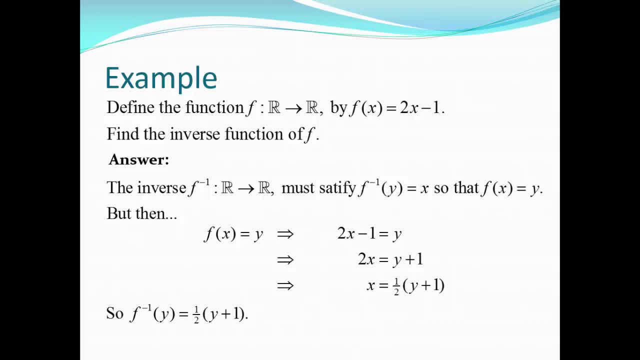 that f inverse of y is x, and that means that f of x must be y. Using that, I should be able to figure out what f inverse of y is in terms of y only, and that will give me the mapping. So to do that, if f of x equals y, 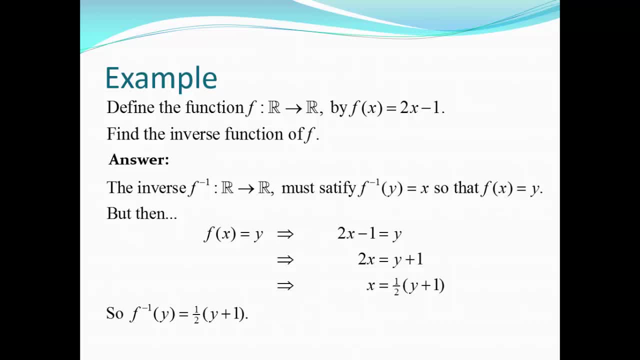 I want to know what x is. That means then: 2x minus 1 equals y. Again I want to know what x is. So I will just solve for x in that equation. I will add 1 on both sides, I will divide by 2 on both sides. 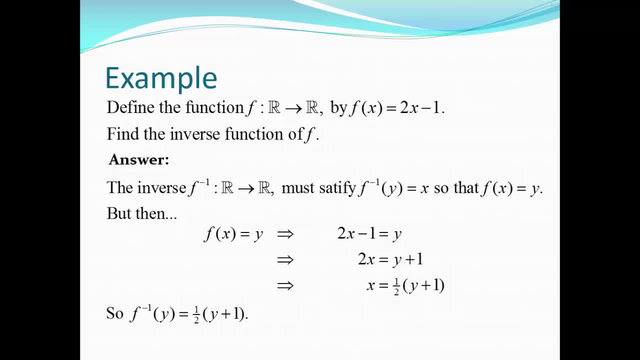 to get x equals 1 half y plus 1.. That is the unique element that y is associated with. So then f inverse of y has to be that x value. It has to be 1 half y plus 1.. So f inverse of y. 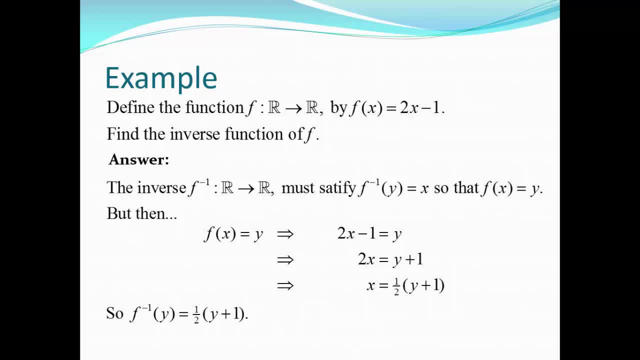 is 1 half y plus 1.. Now you might have been taught in algebra to go ahead and call f inverse and say f inverse of x. I would prefer you don't do that. I would prefer you don't. It makes it actually harder to understand.